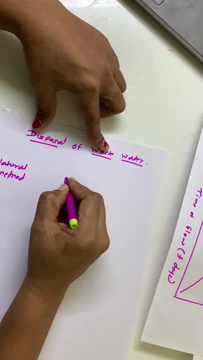 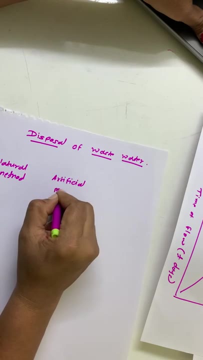 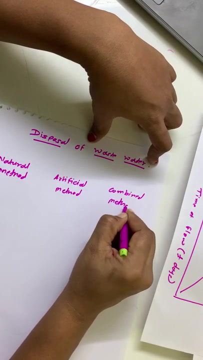 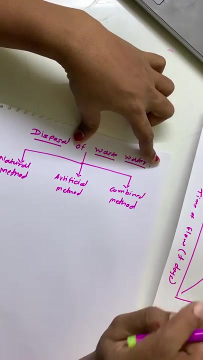 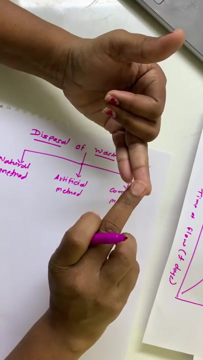 We can say: Second, one is the artificial method And third one is the combined method. So these are the three different ways by which you can dispose the wastewater. Disposal of wastewater: there are two possibilities. One is dispose after the treatment and dispose before the treatment. 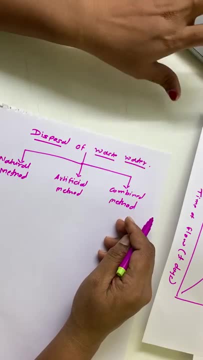 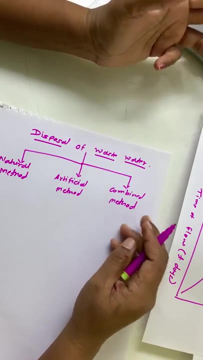 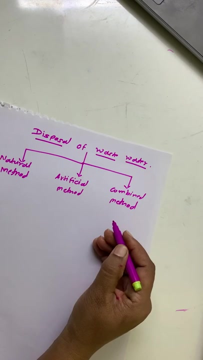 If you have the treatment plant, after the treatment also, you need to dispose it. If you don't have the treatment plant, there is a generation of salt liquid waste from the society and you will have to provide the provision for the disposal of wastewater. Now, first, combine the method in the sense. 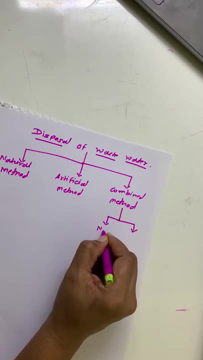 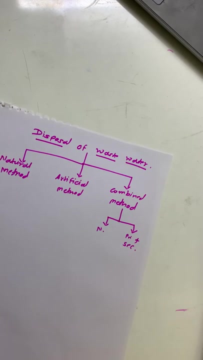 either you can allow to treat the water by the natural way, or you can treat it by using the prime methods and secondary treatment processes, and then you can dispose this wastewater into a near land or the nearby water body. artificial method, in the sense you must give either primary treatment. 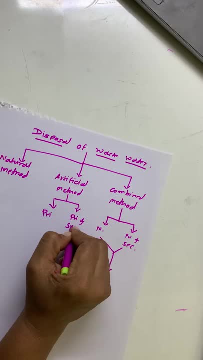 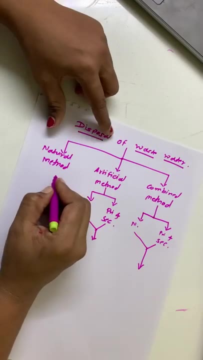 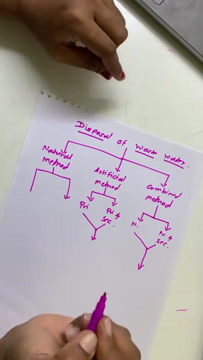 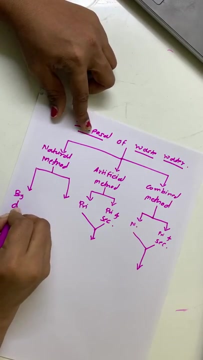 or primary and secondary treatment to the wastewater before the disposal. now the next one is the natural method. i will focus more on this method, as this chapter focuses more on this way to dispose the wastewater. okay, there are two ways: one is by dilution and another is on land. 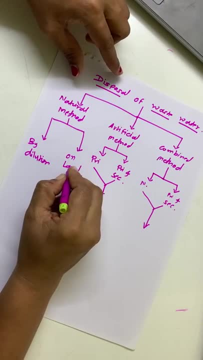 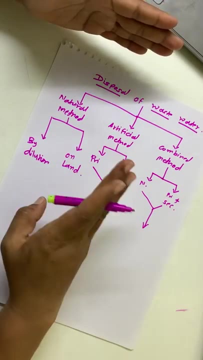 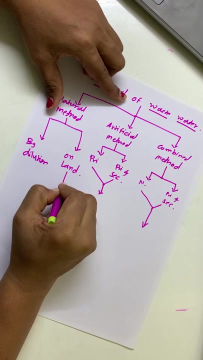 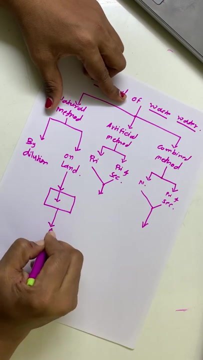 what is the way to dispose the wastewater? why we are going to dispose the wastewater. okay, we want to regenerate the water for the next purpose. is it so on land? when you are disposing it on land, at that time there will be a percolation of water under the ground and it will be collected. 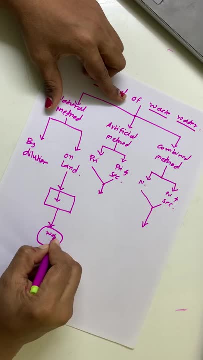 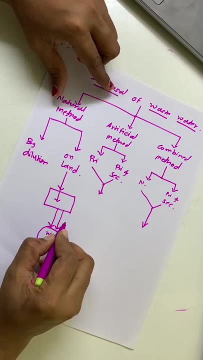 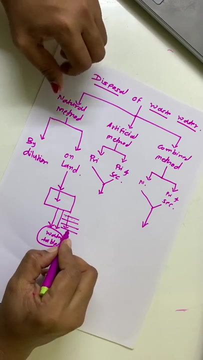 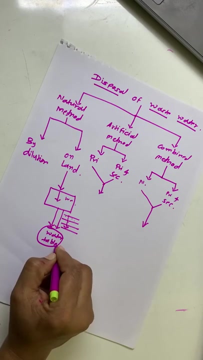 in a underground water table. but when it is passing through this area there are the different layers of the soil. okay, ultimately it is getting filtered out, it is removing the impurities present into this wastewater and then clear water will be collected in a groundwater table. then this groundwater you can. 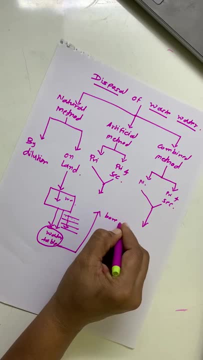 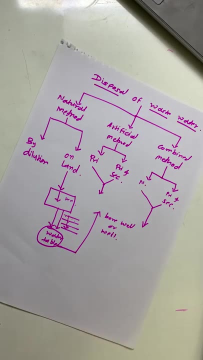 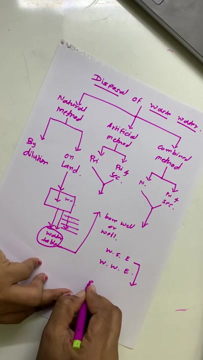 extract by using the bore, well or well, for the regular purpose, or as a raw water source or as a GoPro. so these are the three ways to dispose the waste water. so let's discuss: how do we take it from soil source? we can take from soil the source of this water. we can take it from soil water most more carefully thanks to what we have studied: the disposal of wastewater, our. we have studied the water supply engineering and now we are saying the waste water engineering in a water supply engineering, what we did, we have taken a raw water. is it either from the surface or from the ground? we have gone from this water source fromagens. 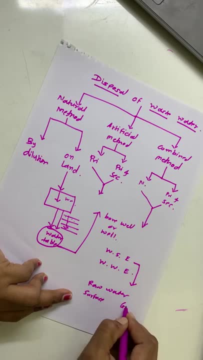 way to dispose the wastewater. groundwater source is it? but this water we are treating by using primary, secondary and some advanced treatment processes, though it is a groundwater, though it is a surface water. if it is the surface water, there are the different sequences of the treatment unit operations. 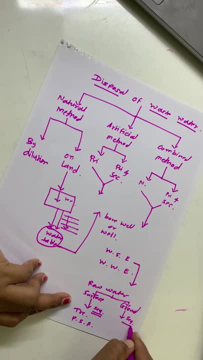 and if it is the groundwater. there are the different sequences of the treatment unit operations and unit processes. but what we used as a raw water, raw water from the surface water body that is, a river or stream or pond, and if it is the groundwater, extracted through the well or 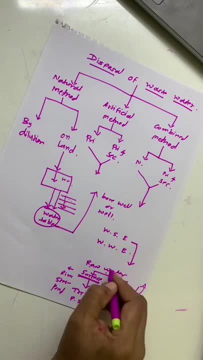 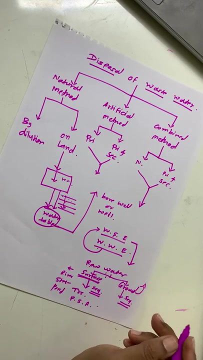 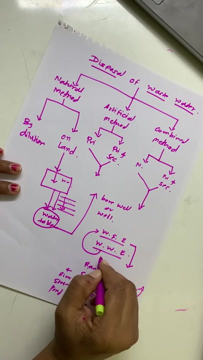 bore well, is it so? this is the raw water we have collected as a raw source for the water supply engineering, Wastewater engineering, after treatment process. it cannot become a water supply, a raw water for the water supply. it has to be treated after treatment, also after treatment of the wastewater. 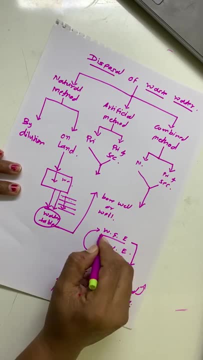 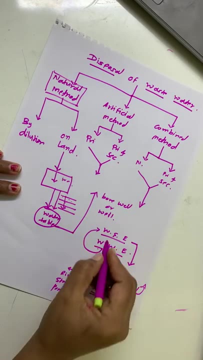 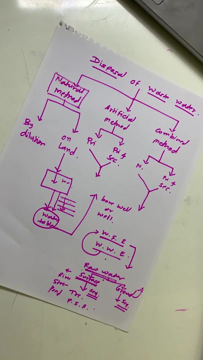 treatment through the wastewater treatment plant. it must pass through the natural method for the treatment and then we can use as a raw water source for the treatment. Have you getting what I am saying? we cannot use the treated wastewater as a raw water source for the water supply. 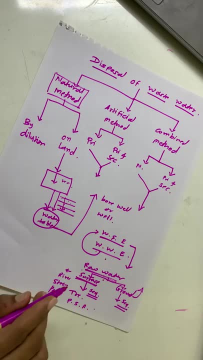 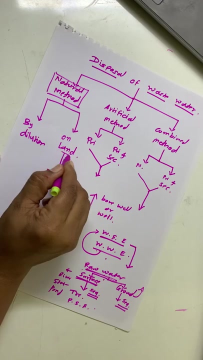 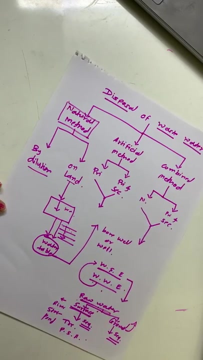 engineering. if you want to use this water as a source for the water supply engineering, you should treat it by the natural method, means you should dispose that water and allowed to treat it by the land or by the dilution method. then only you can use it as a raw water source for the drinking water purpose is. it means what is. 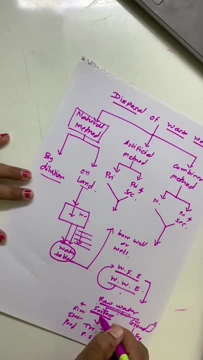 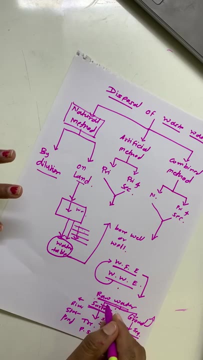 problem. why don't? we cannot use because it has to be treated completely. though we are providing a primary and secondary treatment process to the wastewater, it is not removing the impurities from the water hundred percent. so, whatever the impurities remain after the primary and secondary treatment processes, for the removal of these impurities we have to go for the tertiary. 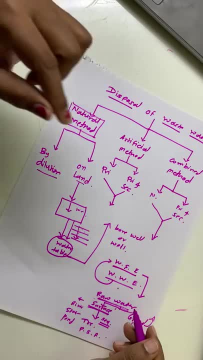 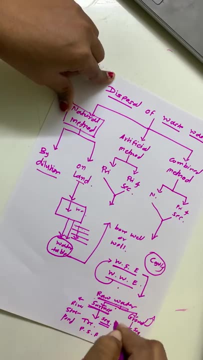 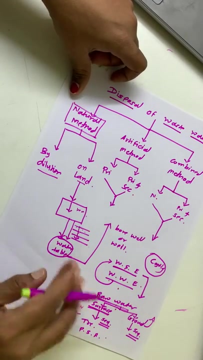 treatment process or the advanced treatment process, and which is very costlier. it will not be a economical process, so that's why we have to give, allow it to get naturally treated and then we can use as a raw water source. so i have explained how to dispose on the land and how we are getting the 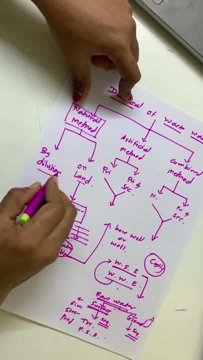 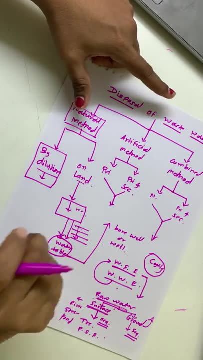 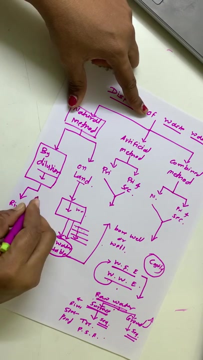 regenerated water through the well and bore well. now i will focus on the dilution method. this is the important part of this chapter: dilution method. dilution in the sense, what we can do. we can allow to flow the water either in a river, either in a stream or in a 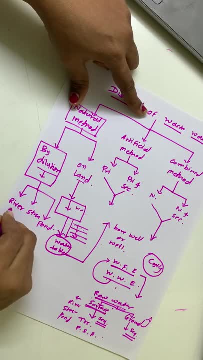 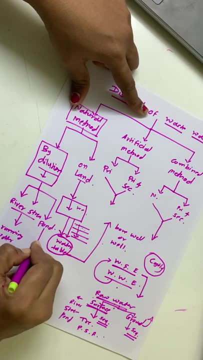 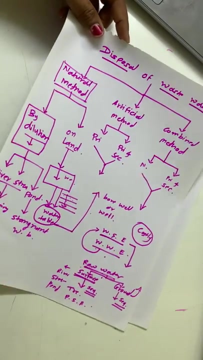 pond. these two bodies can be identified as a running water bodies and this will be identified as a stagnant water body. okay, so treatment in this and treatment in this will be in a different manner that we will see one by one. so this is the little background about the disposal of wastewater. 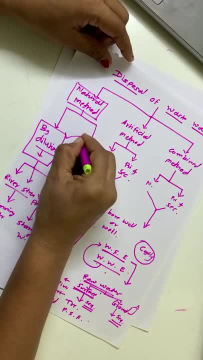 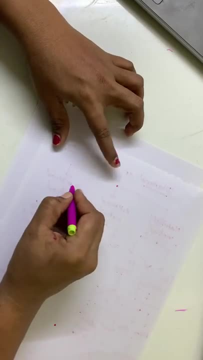 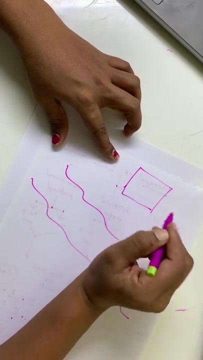 now we will see how, how the water is getting treated by the dilution method. what is mean by dilution? dilution in the sense i can say: suppose this is the stream or the river and this is the one of the village, or we can say a town, and from that 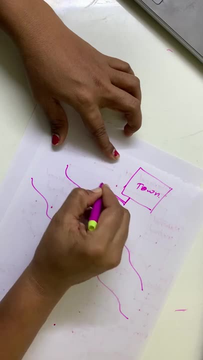 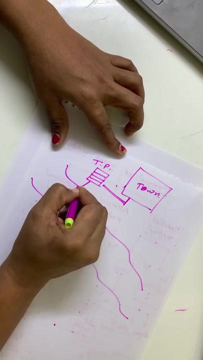 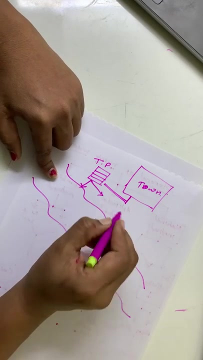 a amount of wastewater is getting generated here. they may have been provided a treatment plant and after treatment they have to dispose that wastewater into the near word by water body, or if they want to dispose on the land, they can give it to the farmers for irrigation purpose. 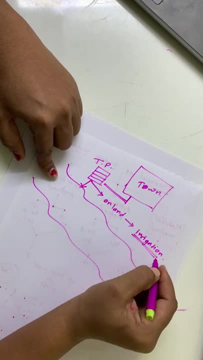 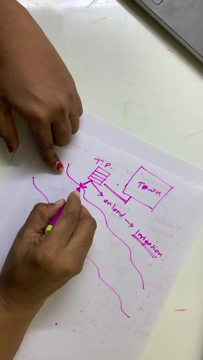 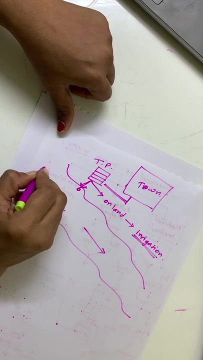 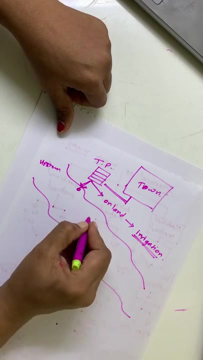 and while percolating on the in the ground, it is naturally getting treated okay. so just focus upon this point. when you are disposing at this point wastewater, the direction of flow will be this: above that part is known as the upstream, and from that point to the next area can be called as the downstream of the river, the moment you are. 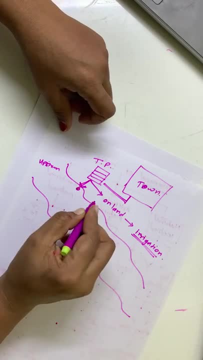 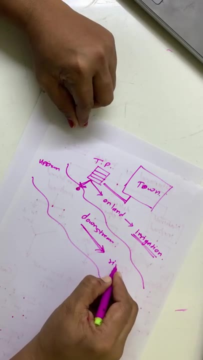 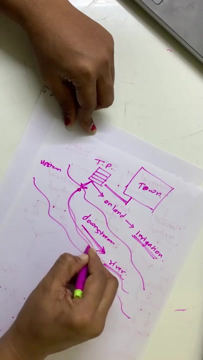 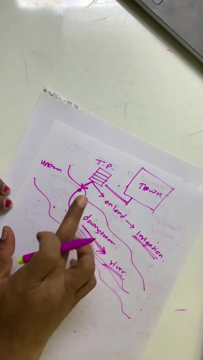 disposing the wastewater into this river water body, it will start degrading the quality of this existing river water but, naturally, how this water is getting treated along with the new water coming into this waste river that we are going to see in this chapter. okay, now, when you are disposing such 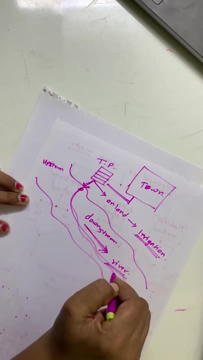 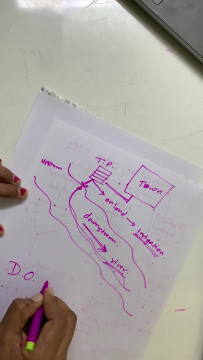 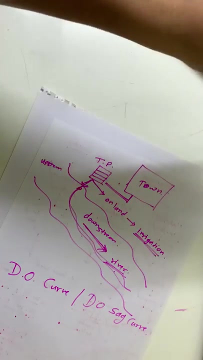 at a particular point. then how the water is getting treated, that i will tell you. there is a concept of dissolve oxygen curve, or we can say: do that curve. so what is that devo sat curve. that i will explain you.